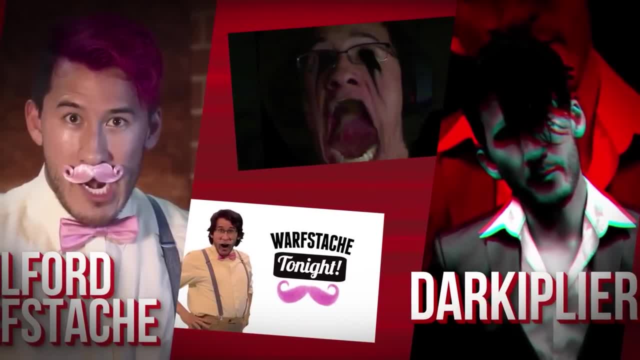 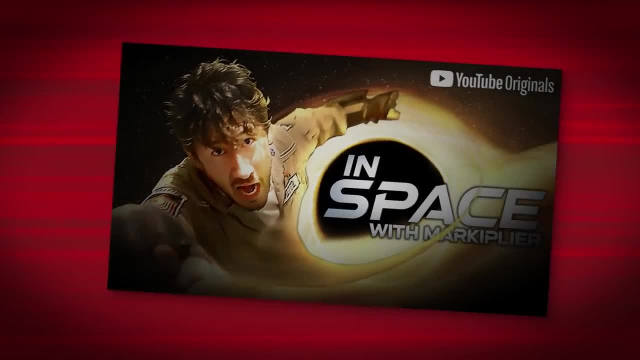 Characters that started off as little one-off jokes that eventually became fully fleshed out with their own backstories and motivations. We've dissected some of this lore before, but with In Space Part 1 being Markiplier's biggest and most ambitious project ever, 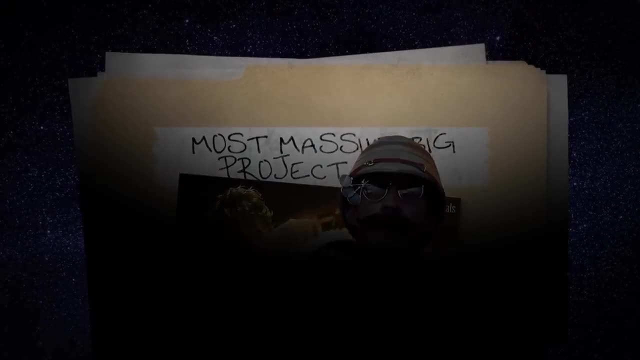 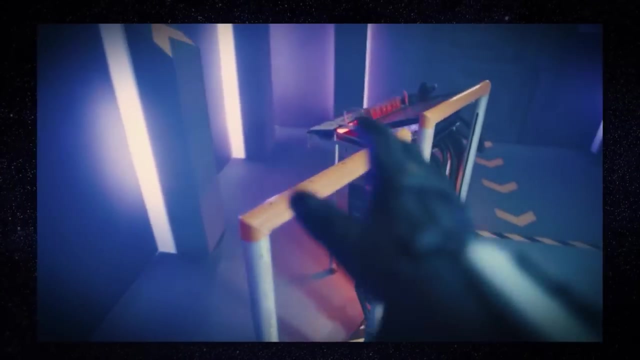 I suspected that these personalities might be making a return. Sure, you can play through In Space to kill off Mark as many times as you want, Totally fine. if that's what you want to do, great, go for it. But there were also moments that kept setting off my theorist. 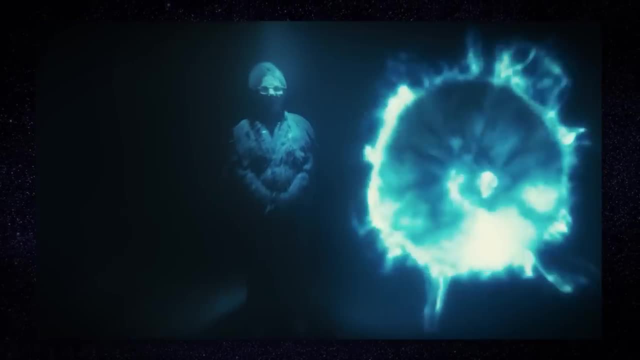 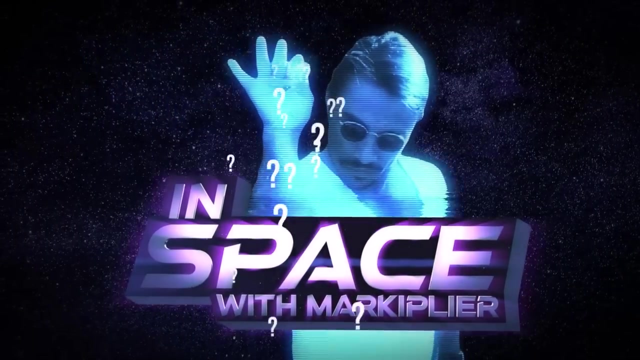 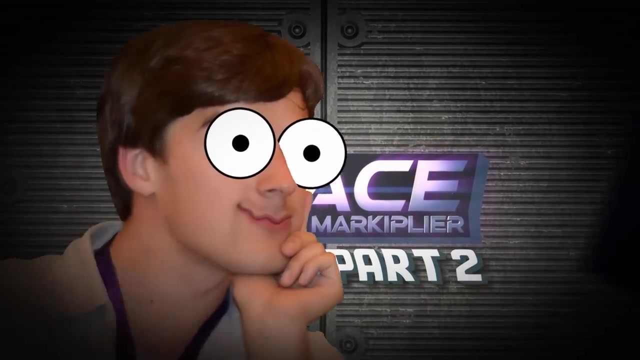 senses, Namely the constant Paradox detected, Or one-off lines that seemed to imply a greater history to this world. Lines like Sprinkled throughout told me that there was a mystery here, A big reveal waiting in the wings to happen in Part 2.. So I dug in And let me tell ya, there is a lot hidden. 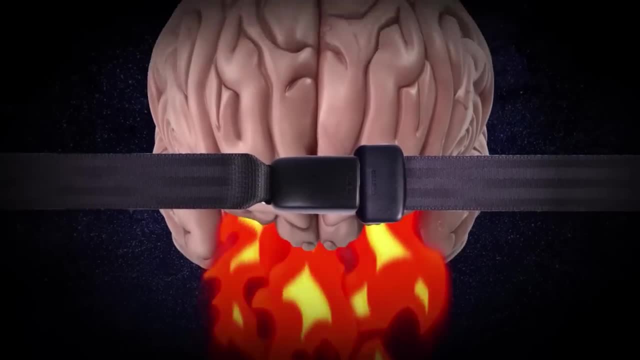 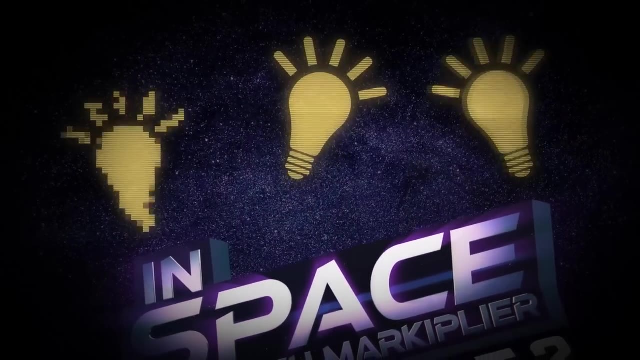 here. Buckle up theorists, cause I'm about to launch your brains into the stratosphere. I think I've figured out what the main climax of In Space, with Markiplier Part 2, is gonna be, and, despite all the hints that Mark's been throwing out, I don't think it's what. 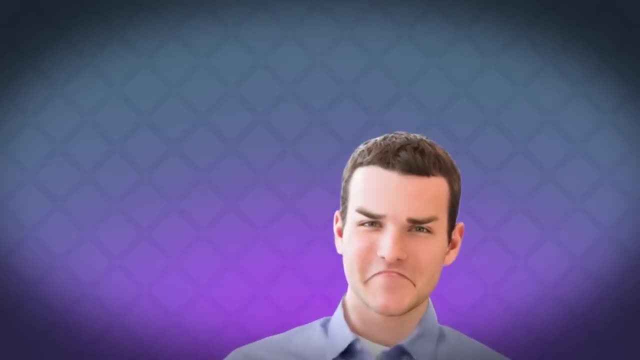 you'd expect. Also, Before we get to the main climax of In Space, with Markiplier Part 2, I want to remind you Before I get too deep into this. I'm sure some of you are thinking that I've cheated, That I'm gonna spoil the ending because I was in the show. The truth is I wouldn't. 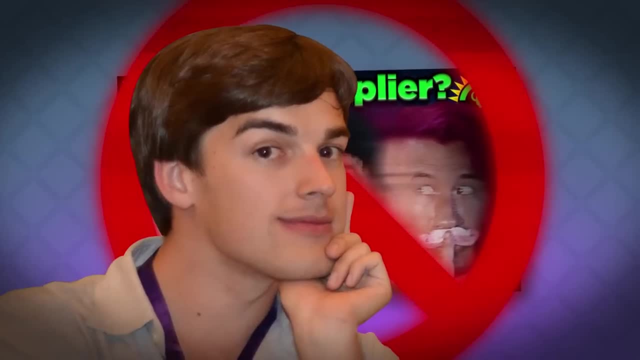 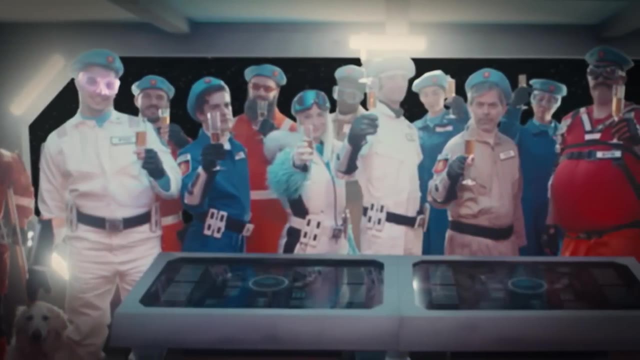 be making this video if I did know the ending. Mark is a good friend and he's worked really hard on this project. I wouldn't want to ruin the surprise that he has for his audience When working on the show. I never saw the whole thing. I was only exposed to the parts. 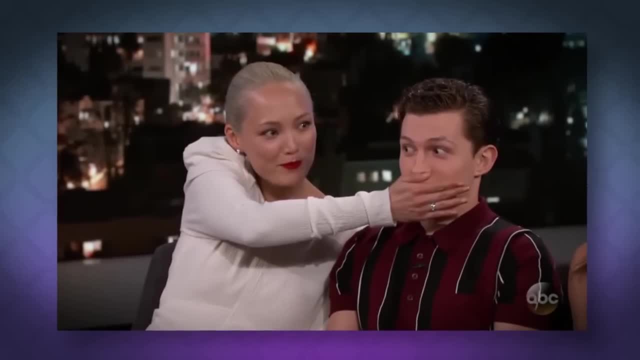 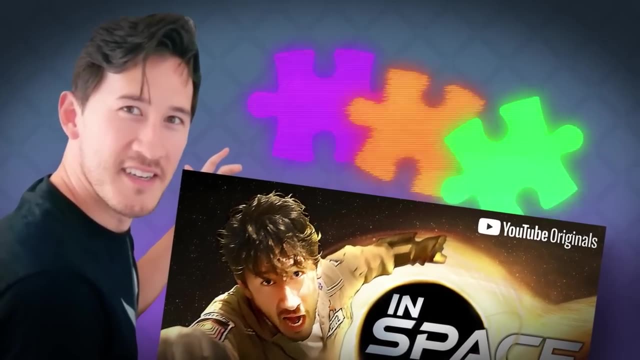 that I was in TLDR here. I don't want to act as the Tom Holland of this MCU Markiplier Connected Universe. This is being treated like any other video that we do. We're dissecting clues that are presented within the videos that we have at our disposal, and that's. 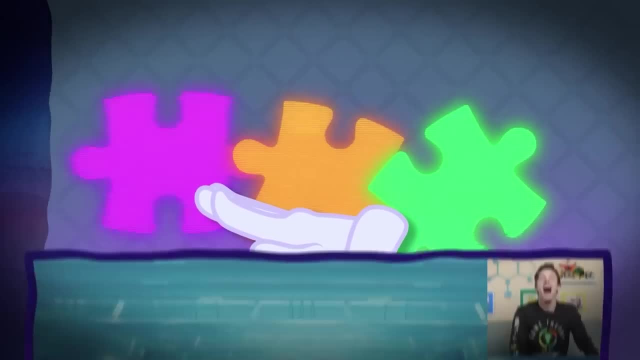 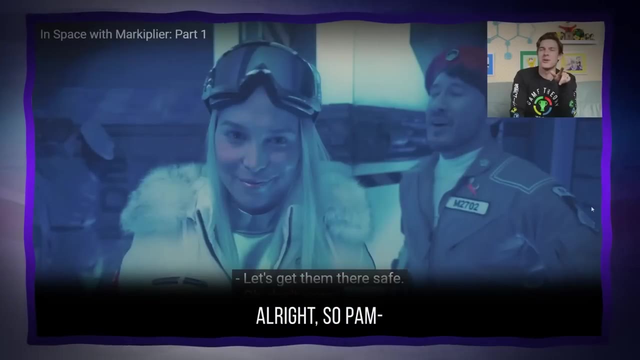 it. We're not pulling from any extra insider information. So in my initial playthrough of In Space on GT Live, I pointed out that we needed to be wary of Celci, the head of Cryo, played by Pamela Horton. Alright, so, uh, Pam, always important to note with these episodes, as we've done in. 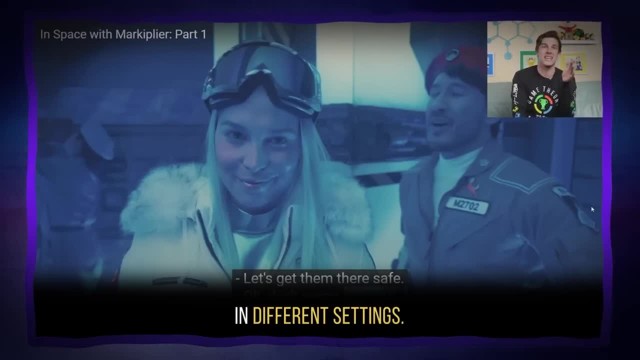 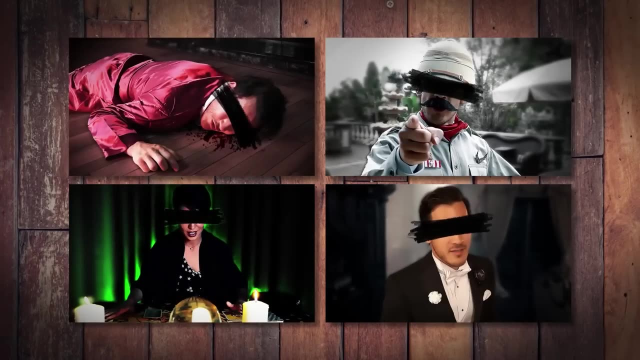 a previous theory. Pam tends to be the same character in different settings. You see, Pam's most notable character to date has been Selene from, Who Killed Markiplier, a four-part murder mystery released back in 2017.. About a friendly poker night that goes south, And when it comes to Markiplier, lore this. 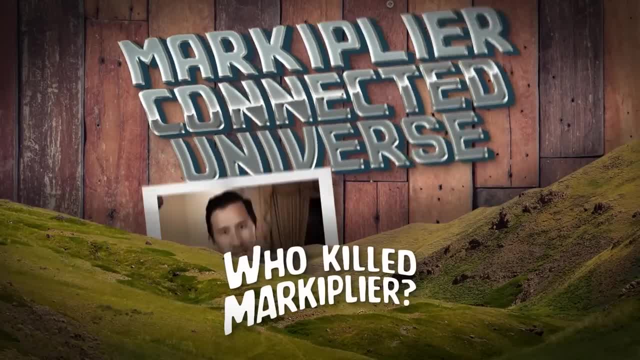 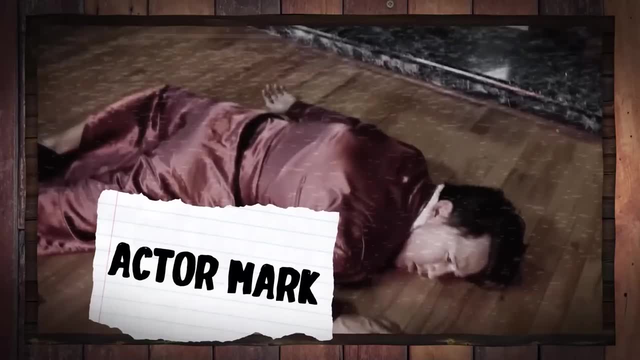 series really is the foundation for his MCU, as it provides us the backstories for pivotal recurring characters In it. a pompous jerk named Actor Mark dies Yep- that is officially what he's known as in the canon- And the primary suspects include his childhood friend. 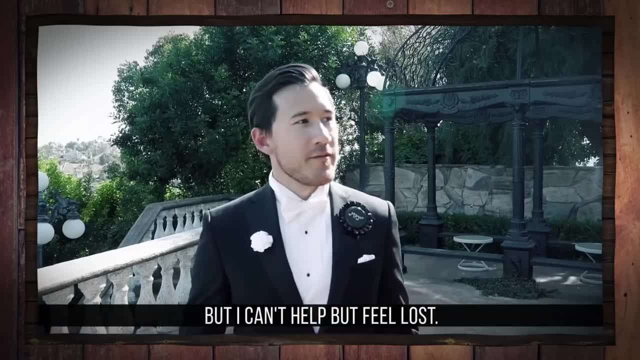 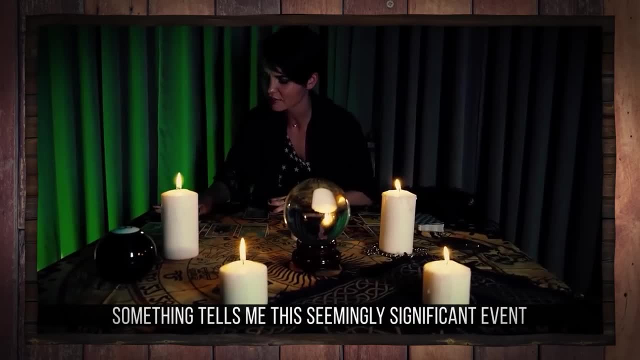 Damian the mayor. I know I'm supposed to be a leader in this scenario, but I can't help but feel lost. Damian's sister and Mark's ex-wife, the mystical Selene. Something tells me this seemingly significant event is actually a. 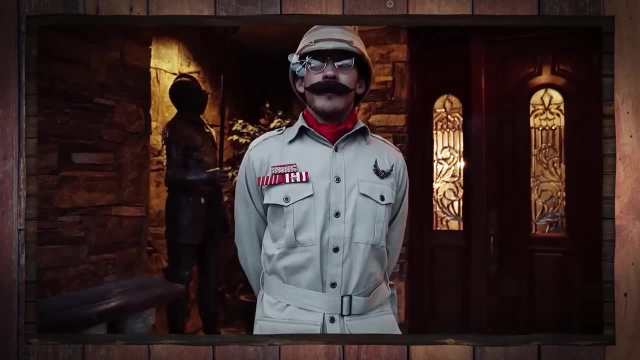 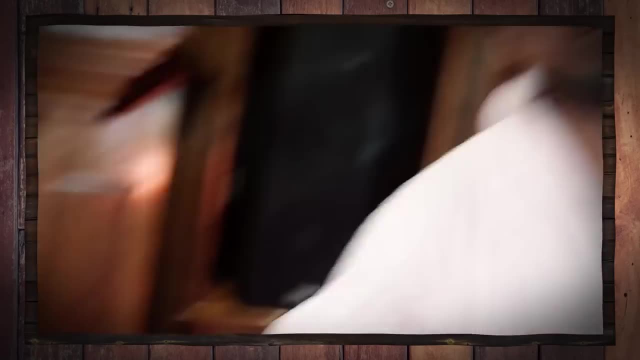 footnote in a much larger mystery unfolding in our midst. And the wacky mustache-twirling gun-toting colonel. Life needs a bit of madness, eh, chap, It turns out Actor Mark's death was all part of a greater plan, Thanks to some magic within. 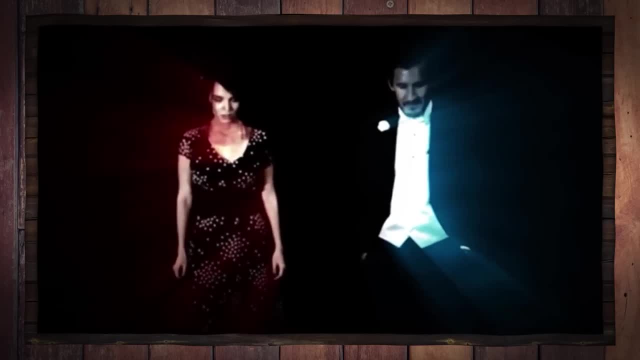 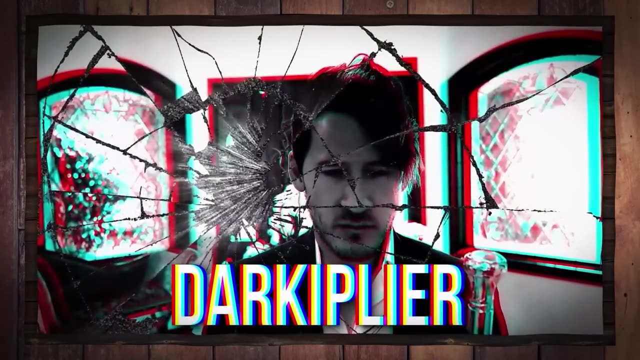 the mansion Actor, Mark is able to take over Damian's body, while Damian and Selene both take over your body, which gives rise to Mark's most infamous character, the red-and-blue-filtered Darkiplier. Meanwhile, seeing his friends die and come back to life takes a bit of a toll on the 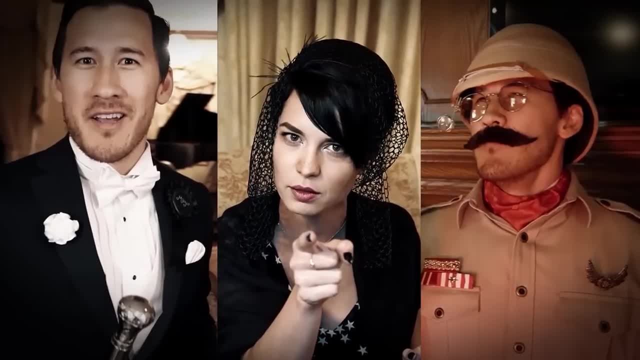 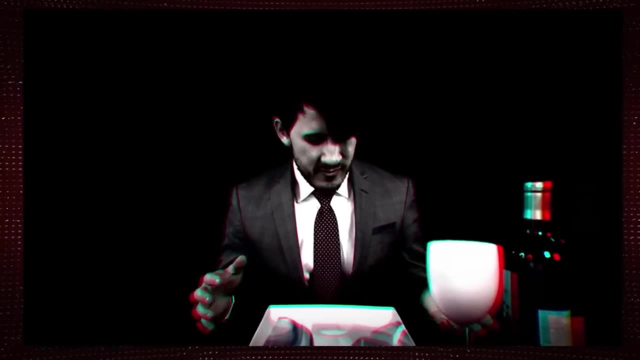 old colonel, Which causes him to go mad. All these characters then recur throughout Markiplier's other narrative videos. When Darkiplier suddenly shows up in an ending of A Date with Markiplier, we know that he's connected to Damian and Selene. 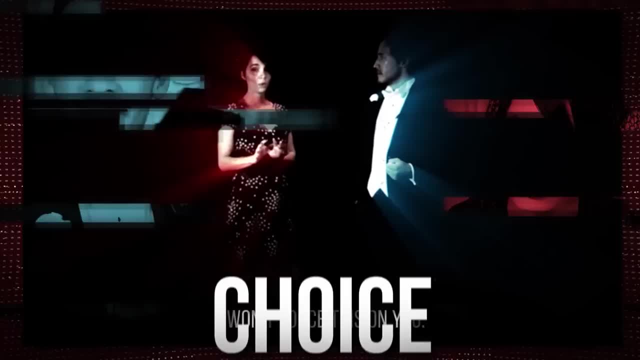 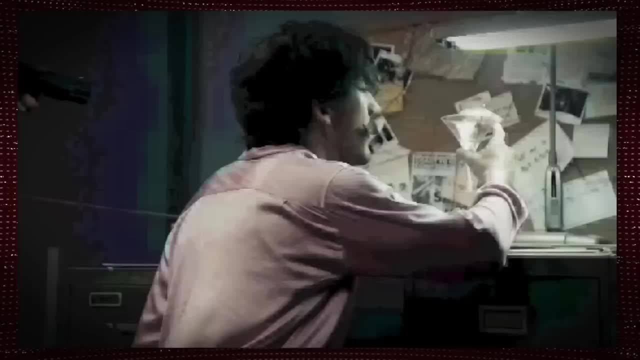 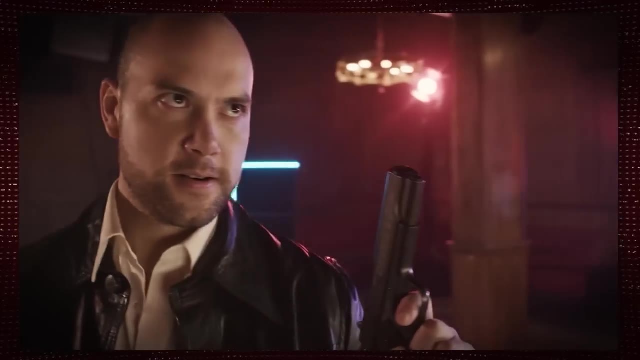 thanks to the same red-blue filter and the recurring theme of choice. I won't force this on you. You have a choice here. I'm tired of giving people a choice. And the colonel story continues in Wilford, Mother Loving, Worfstache, where we see the detective from Who Killed Markiplier hunting down the now deranged colonel. 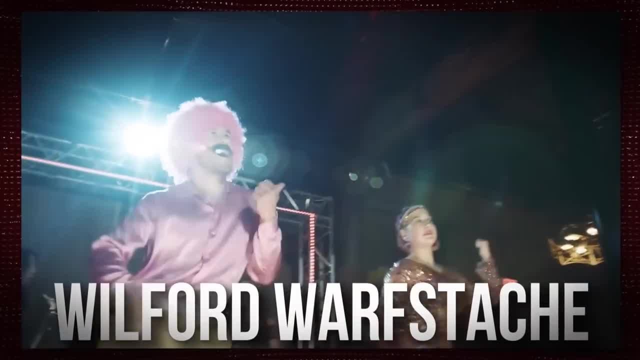 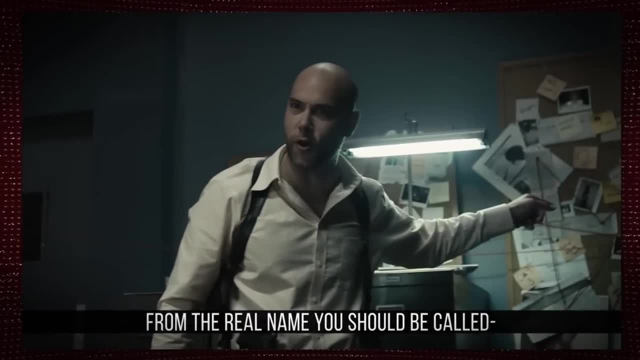 transformed into the reality-warping killer-slash-journalist Wilford Worfstache. Name after name after name, just so you can distance yourself from the real name, you should be called Murderer. Wow, There we all are. 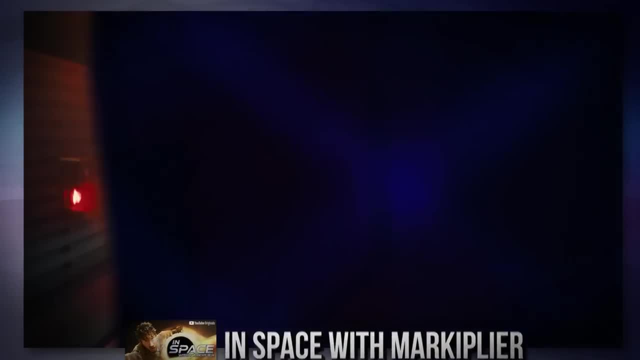 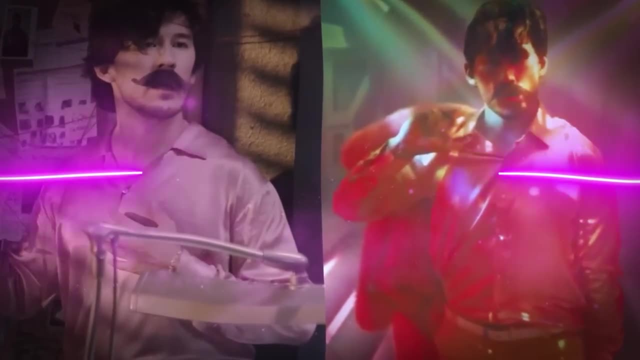 How the hell did you do that? So when In Space features a surprise appearance by Wilford boogieing down to 70s music, wearing largely the same outfit he was wearing in Mother Loving Worfstache, you know that these canons are going to be somehow connected. Given those connections, I did some digging on Pam's new character. 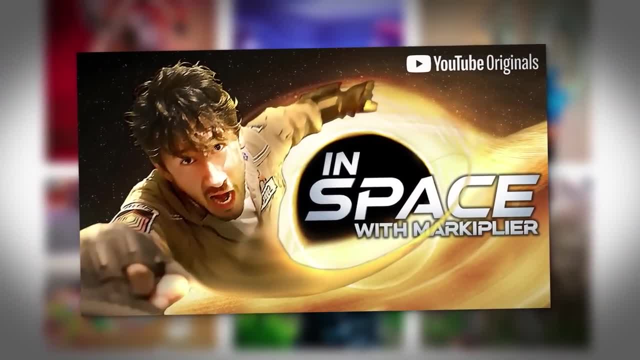 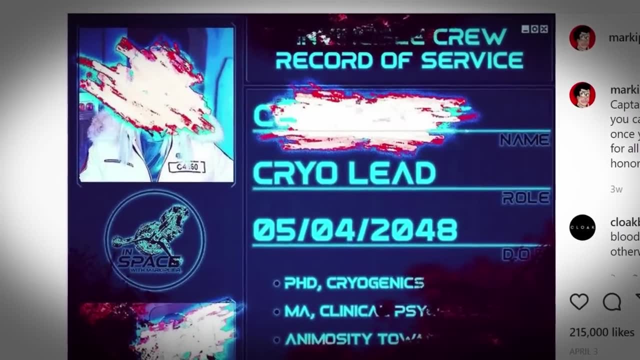 Selsie. Just before the release of In Space Part 1,, Mark posted some photos to Instagram showing the credentials for various crew members aboard the ship: Burt, Gunther and, of course, Selsie. But did you notice anything different about Selsie's card? 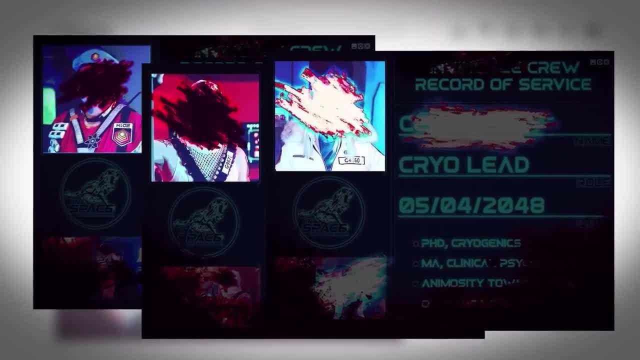 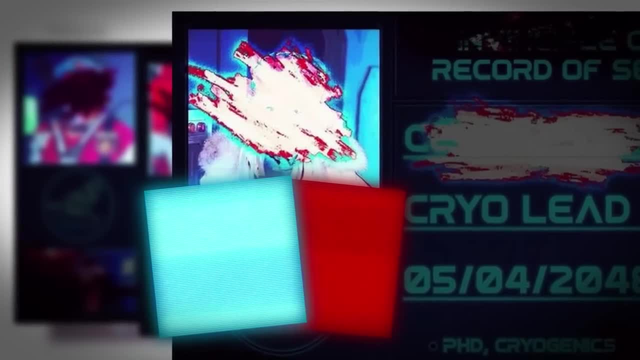 All of them have their faces scratched out, but Selsie's, instead of the typical black, is scratched out in white, with a very distinctive blue and red accent, A motif that's been used time and time again whenever Dark Applier is kicking around. 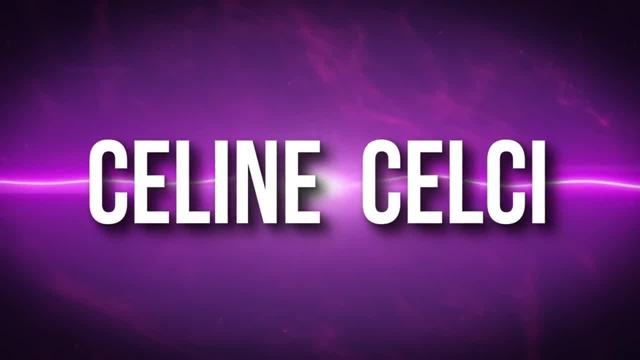 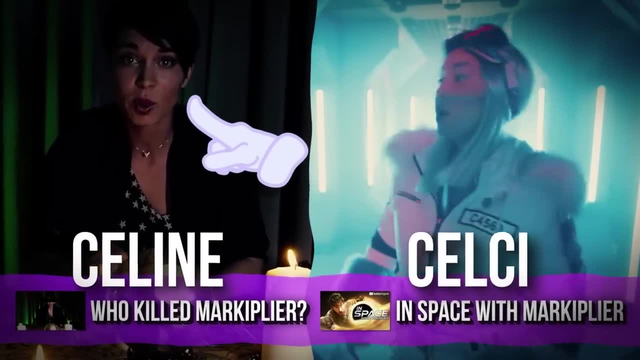 You also very obviously have a name connection: Selsie, Selene- Very similar, So could these two actually be the same character? Could Selsie in this new series actually be the seer Selene from Who Killed Mark Applier? 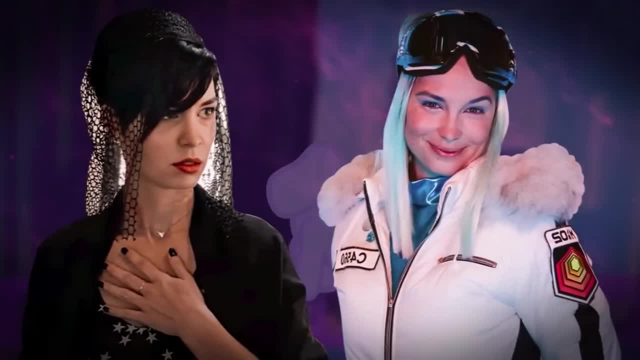 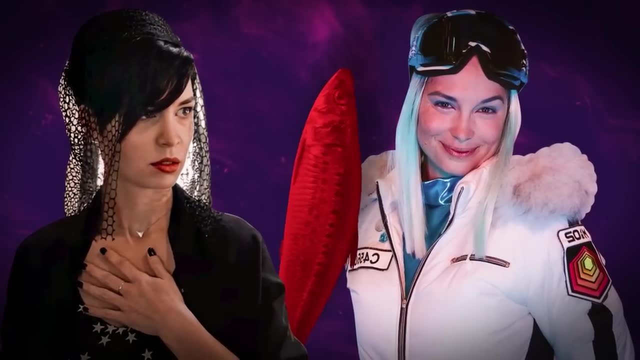 The answer is surprisingly, no. Mark has definitely put some parallels in there, but I couldn't find a linchpin to say that the two were definitely one and the same. So why put in a red herring like that? Well, just because Selsie isn't Selene doesn't mean that Selene isn't aboard the ship. 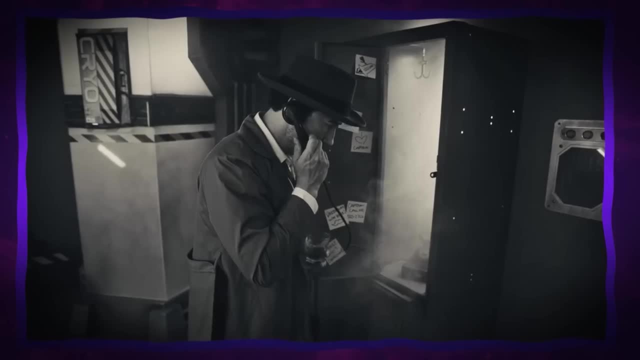 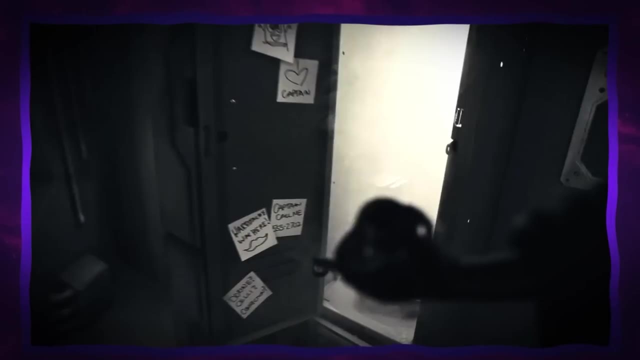 During In Space. if you choose to fire all weapons at the wormhole, Mark opens a locker. that's covered in post-it notes. You've got references to Tiny Box, Tim Worf's stash, Mark's undying love for the captain. but take a look at the bottom post-it. 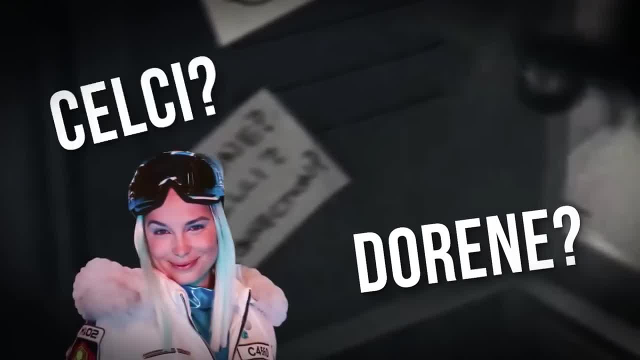 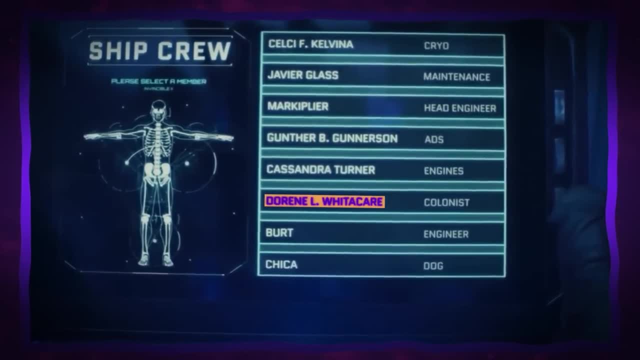 It says Doreen-Selsie connection. Okay, we've talked about Selsie, but then who is Doreen? This one's not super complicated. On our tablet we have a list of crew members with the name Doreen L Whittaker on it. 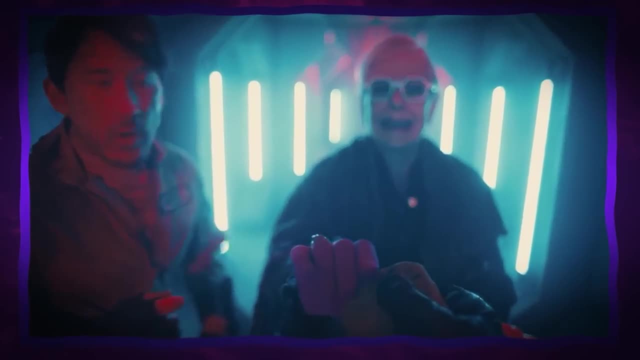 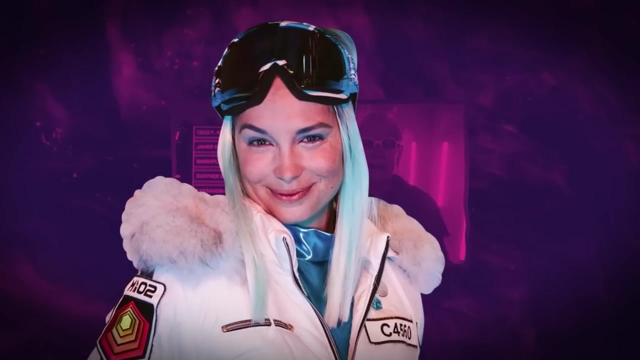 Later, when an old woman glitches into reality to offer us some cookies, Mark refers to her as Mrs Whittaker, So I think it's pretty safe to say that they're one and the same. But what does that have to do with Selsie? 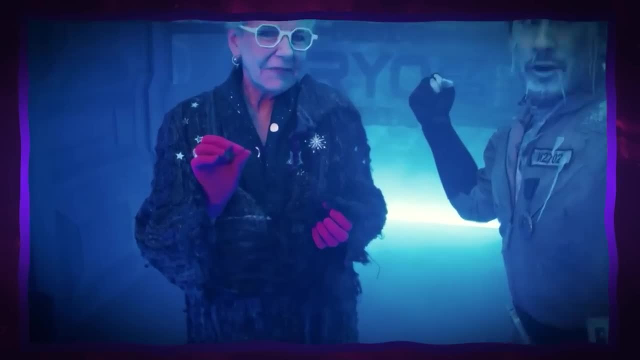 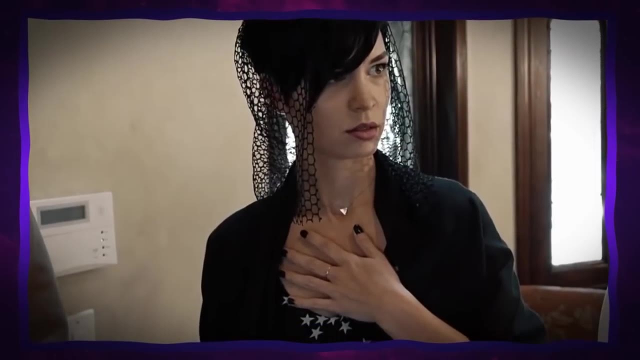 Or Selene for that matter. Well, take a look at Doreen's clothes. The outfit Doreen's wearing is a flowy black dress covered in a celestial pattern- Stars, planets, that kind of thing- Which is incredibly similar to the dress that was worn by the mystical Selene throughout Who Killed Markiplier. 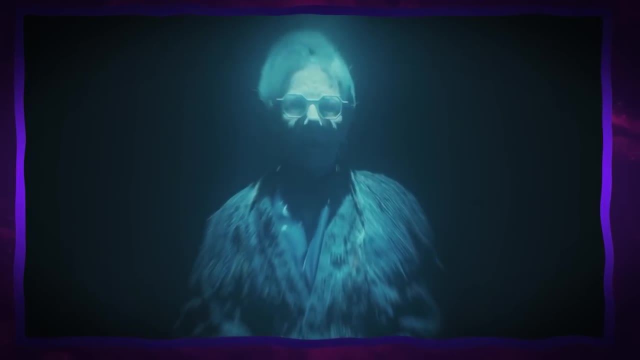 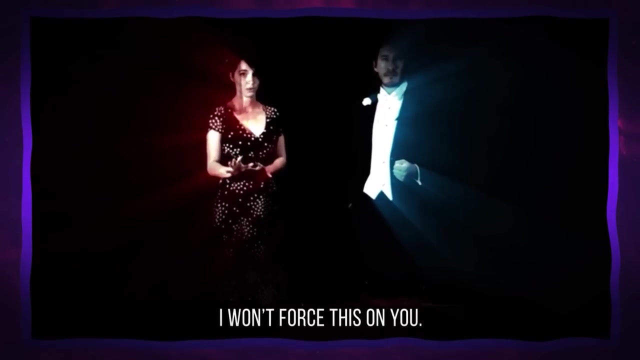 But that's not all. In one of the secret endings, Doreen appears and says some very familiar sounding lines. That's your choice. You always did have a choice. I won't force this on you. You have a choice here. 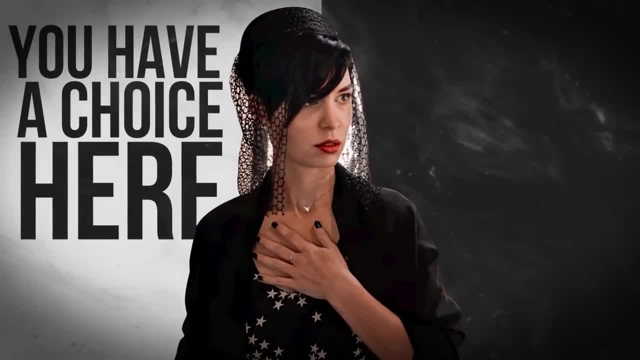 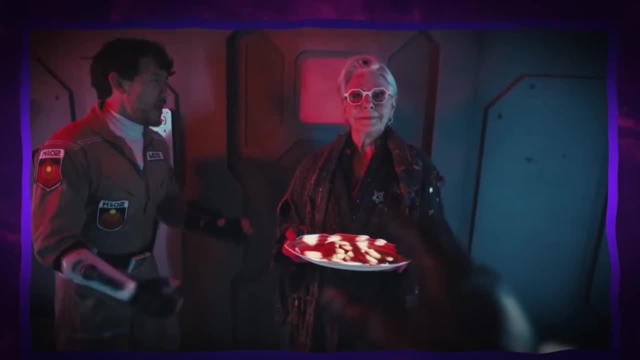 Selene, as a character, has always been about choice, Talking about giving us a choice Or a lack of choice that we have. So it's important that Doreen is saying these exact same things And finally, Doreen gives us this very important line: 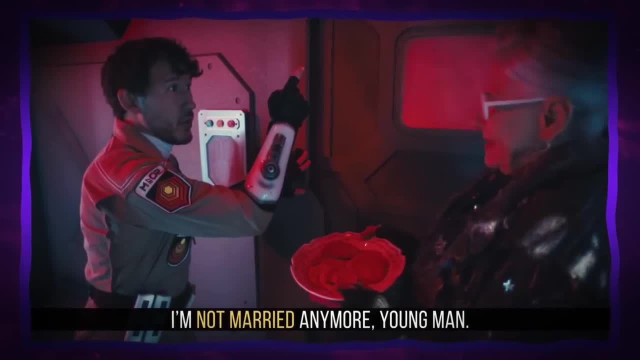 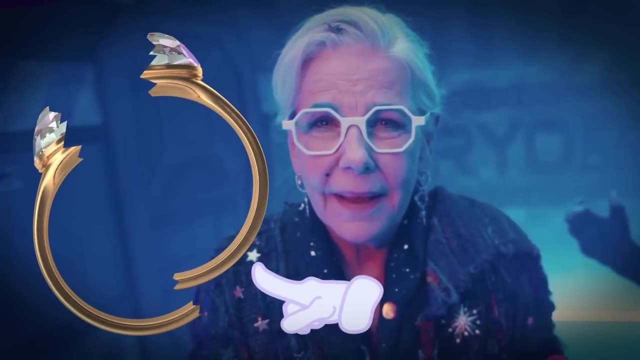 So, Mrs Whittaker, we need you to get in the ass right now. I'm not married anymore, gentlemen, A fact that gets repeated a couple times. I told you: I'm not married anymore. Why make us so aware of this detail, about a seemingly random character? 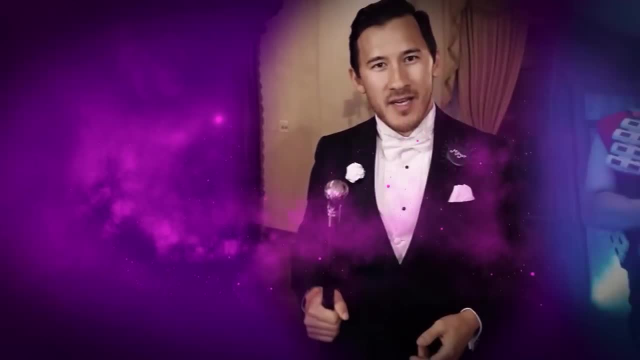 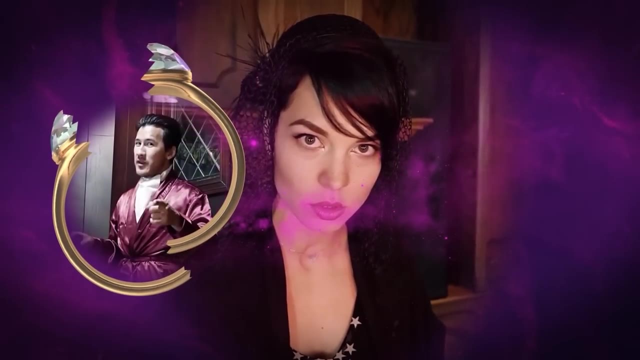 Well, it's designed to point us in the direction of another character. we know, The only other main character within the franchise to be divorced, Selene. She was divorced From the actor Mark in Who Killed. In short, Selesee was the logical stepping stone. 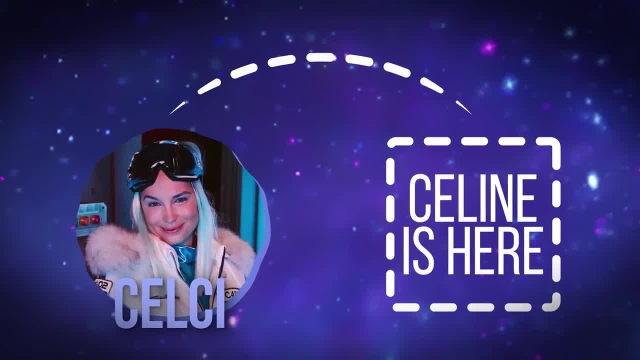 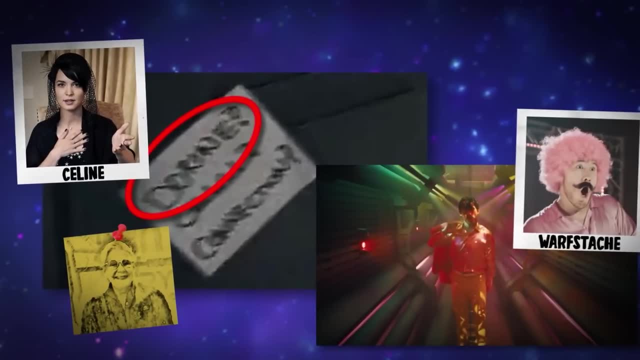 A hint from Mark to us theorists that Selene was in fact here, Just not in the body that we expected her to be in, Not in Selesee, but in Doreen. So Selene is here and Worfstache is definitely here. 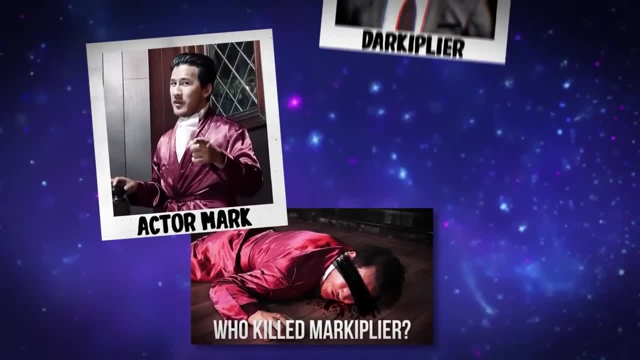 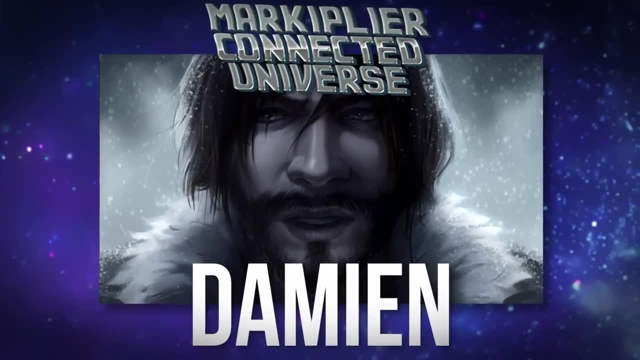 Then, where are the other characters from the story? Where are actor Mark and, most importantly of all, Dark Applier? Well, back in May of 2019, Mark released another video as part of his Mark Applier connected universe Damien. 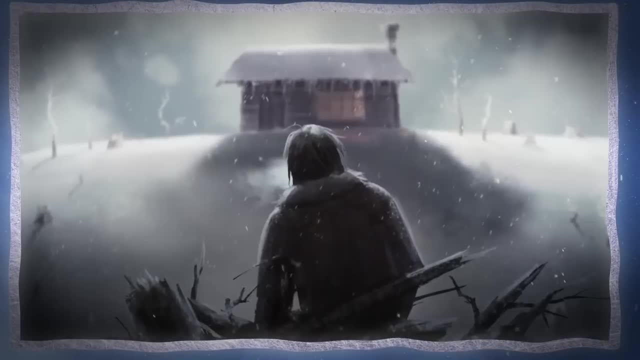 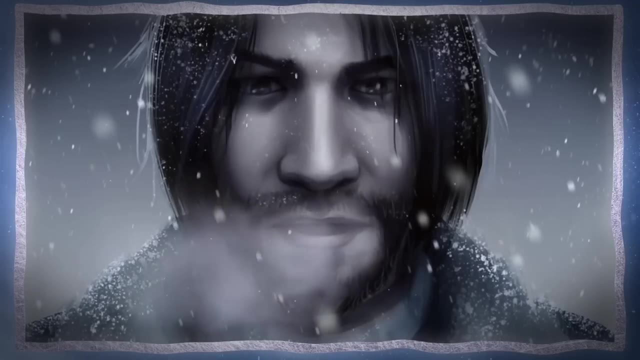 This video, if it wasn't obvious, focuses on the character Damien And the frosty limbo that he and Selene exist in after the events of Who Killed Mark Applier. In it, we see Damien going through a looping cycle, day after day, until his routine is broken by the evil actor Mark. 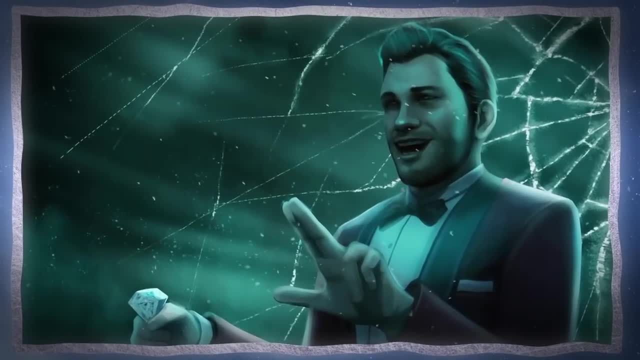 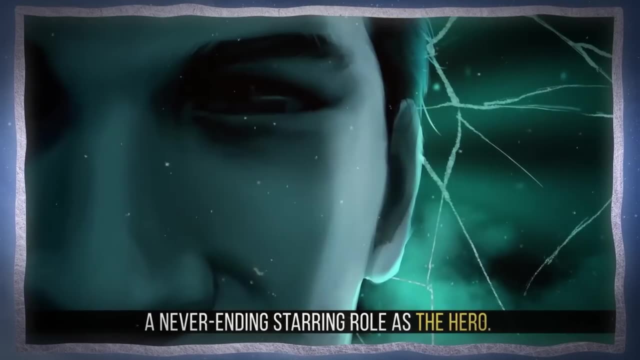 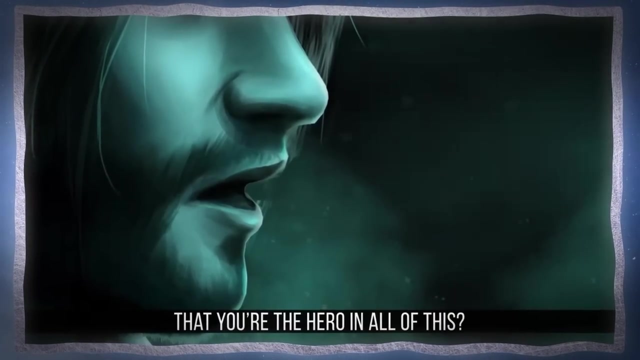 Narcissistic as ever and obsessed with having someone play the villain to his hero. You don't realize. this place is a dream, A never-ending starring role as the hero. But what is a hero without a villain? You honestly think that you're the hero in all of this. 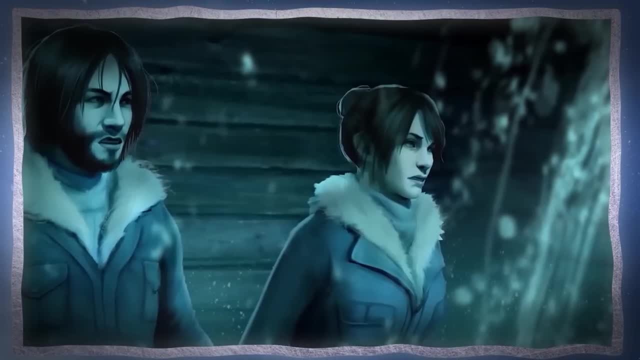 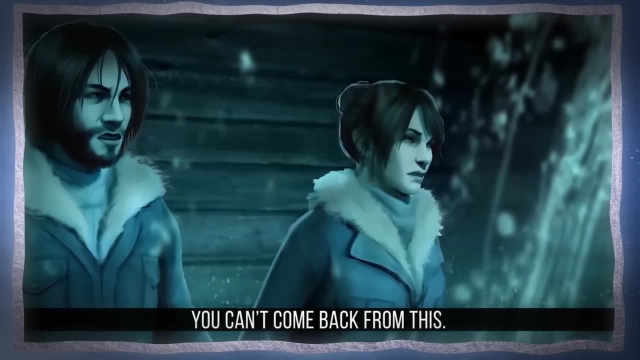 Well, of course I am. In the end, Selene cedes control of Dark Applier to Damien alone so he can get his revenge on actor Mark while she goes to rest. You can't come back from this. It'll change you. 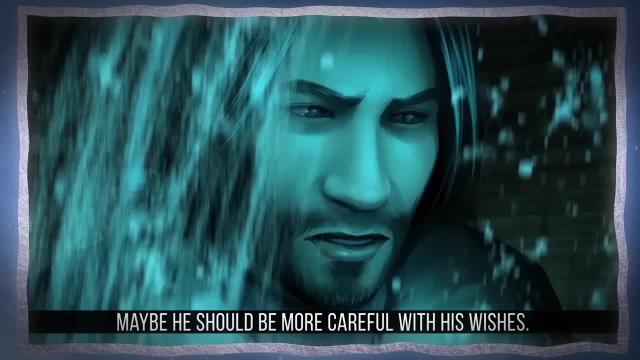 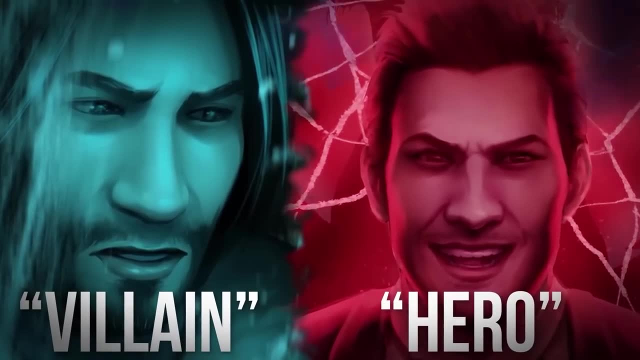 Well, he did say he wanted me to be the villain. Maybe he should be more careful with his wishes. Notice the language here, This repeated emphasis on the battle between a hero and a villain. Now look at In Space, Part 1.. At the start of the story, when we're introduced to our head, engineer and primary Mark. 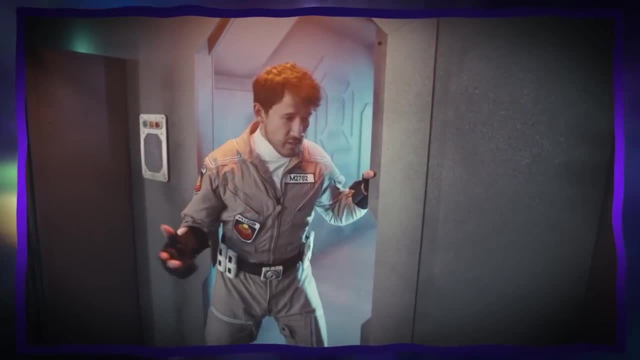 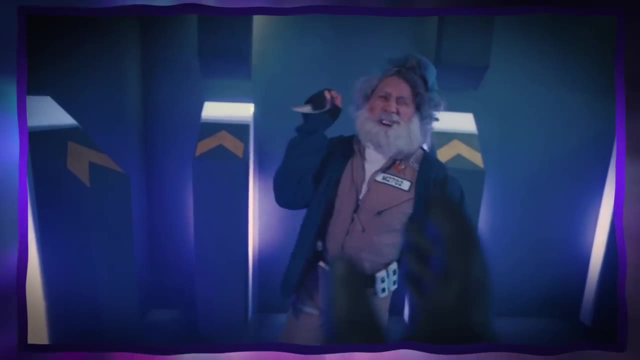 he gives us lines that seem to imply that we go way back, Just like old times here, Captain, And then later in the majority of the endings, we're confronted by an old version of Mark One, who again seems to share a long history with us. 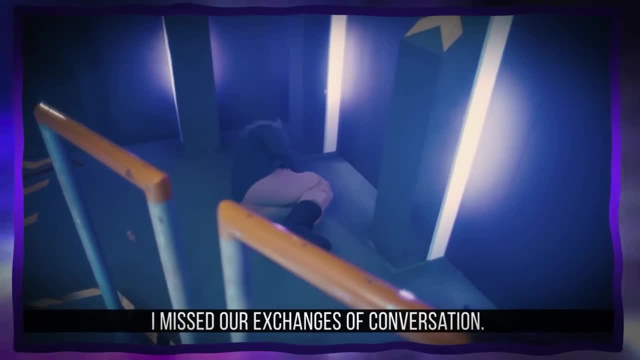 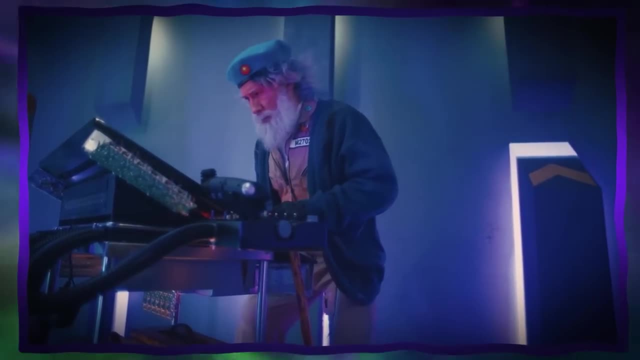 Friend of mine, Oh, close confidante, I'm hysteric, Dangerous of conversation, One who apparently has something to apologize for- I'm sorry about a lot of things- And someone who's been waiting a long time to try and stop our apparently evil plans. 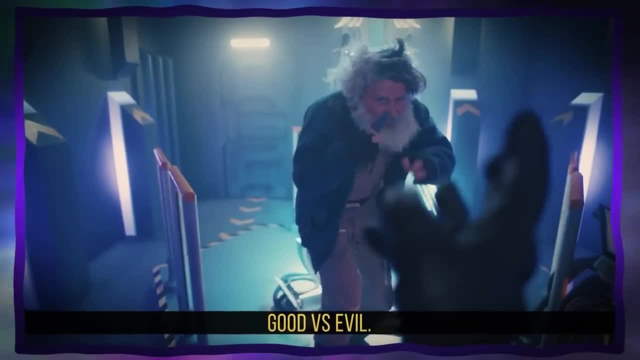 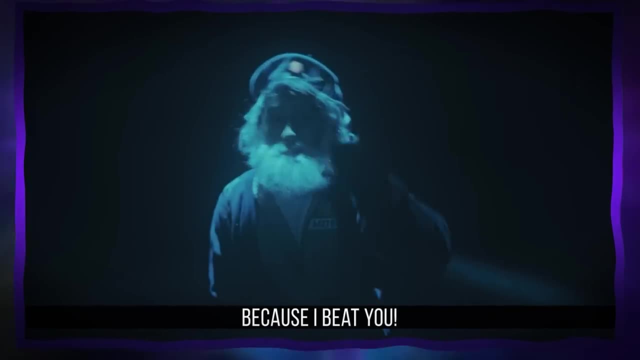 I can't let you win. This is the final confrontation, Good versus evil. This is the villain. When he succeeds, he tells us that it's time to move on. It's all in the past Because I beat you. It's weird. None of this seems to fit. 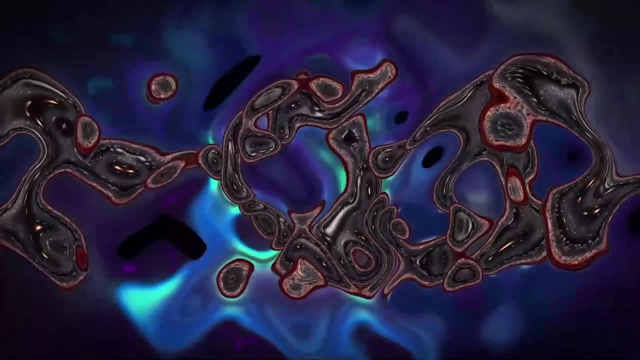 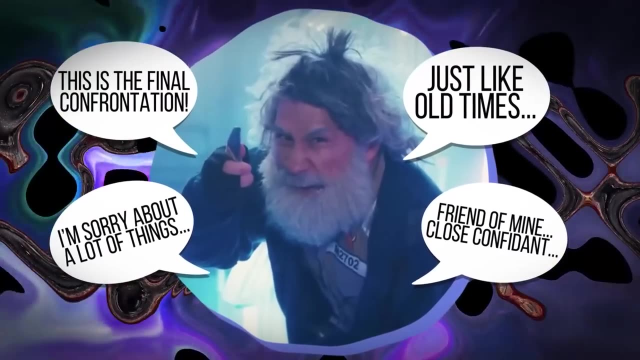 Like. I know that we screwed up the multiverse via our choices as the captain, but it doesn't seem like this is the way that this character would respond. Seems like he's commenting on things that are outside of the story that we were presented. 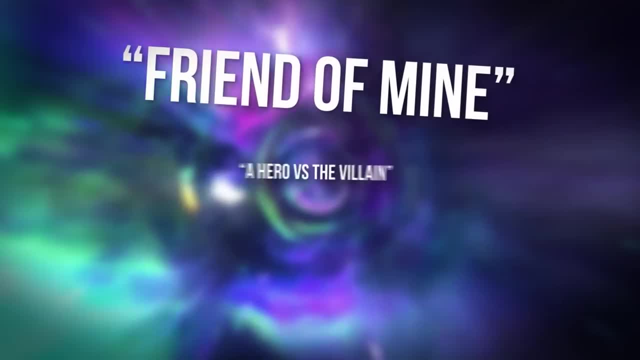 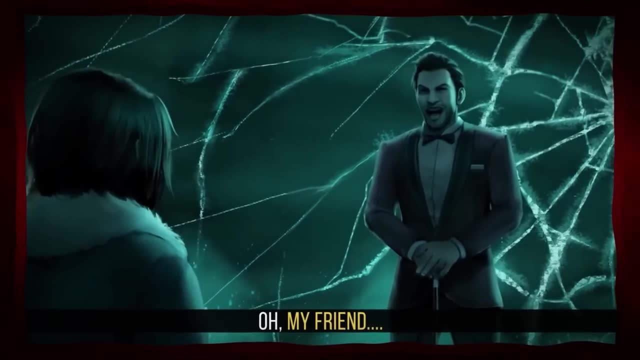 And he is. The thing is, we've seen one character say all of these lines before Repeat all of these same ideas. Friend of mine, Oh close confidante, Oh my friend, It's all in the past, But that's all in the past. 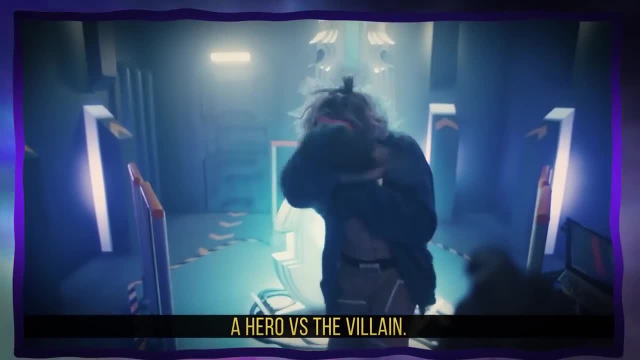 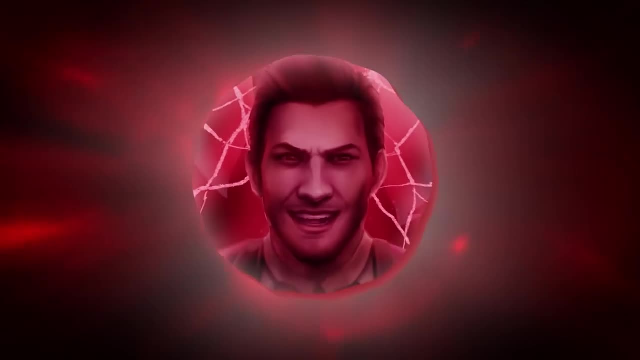 Good versus evil, The hero versus the villain. But what is a hero without a villain? This isn't just any Mark. this is actor Mark. He's now in the role that he's always dreamed of. He's the hero. He's the one that gets to save the multiverse from evil. 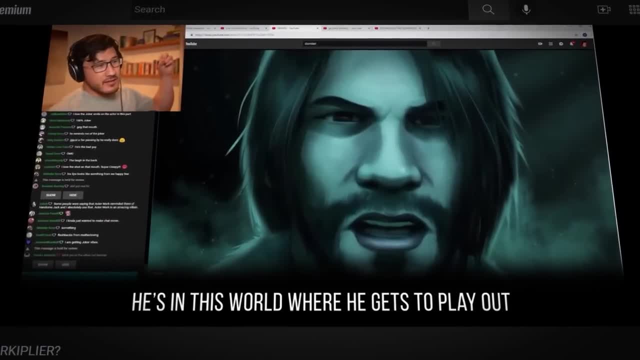 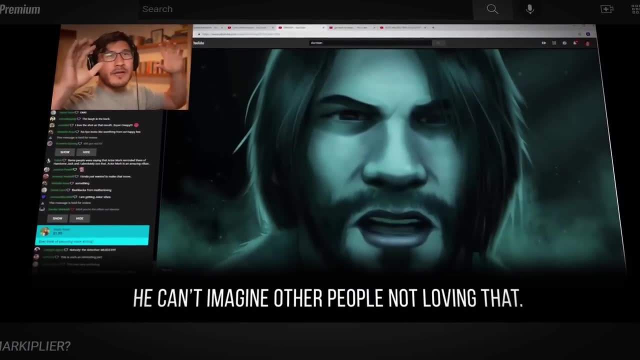 Mark put it like this during his breakdown of Damien: He's in this world where he gets to play out the leading role of any story he wants. He can't imagine other people not loving that. He's just a narcissist. He can't even imagine that he's wrong. 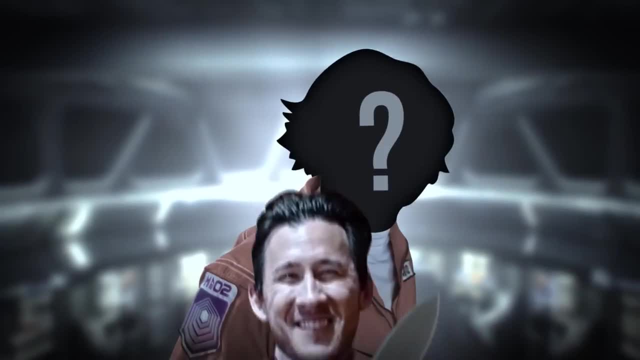 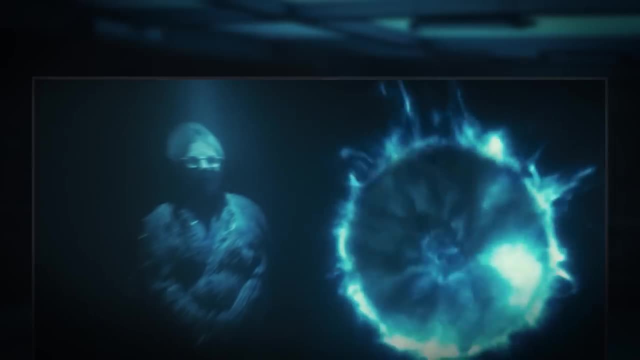 But then why is Mark so determined to defeat us? It seemed like the captain was meant to just be us, the viewer, put into this adventure, But I'm not entirely convinced that that's the case. Even Doreen has us questioning our identity. 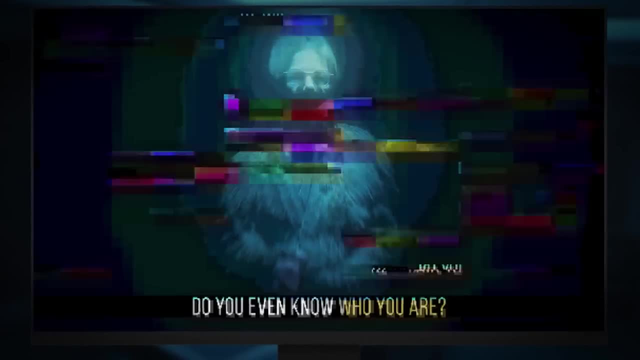 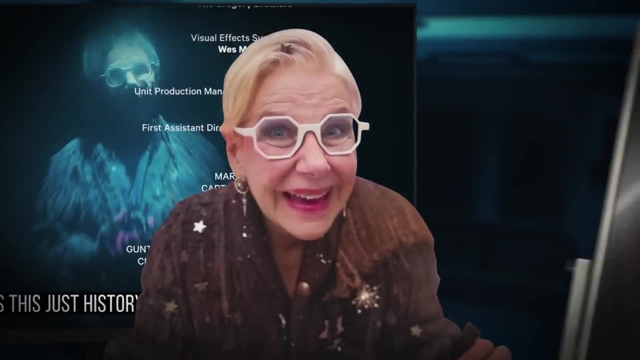 You can't say: I'm surprised. You always were stubborn. Do you even know who you are? Do you feel like you've been here before, Or is this just history repeating itself? She knows us. We are Damien. We are Darkiplier. 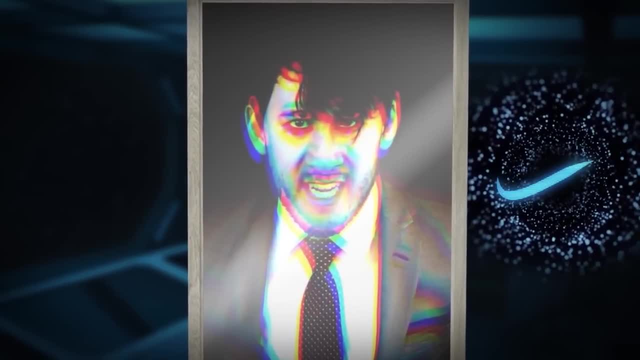 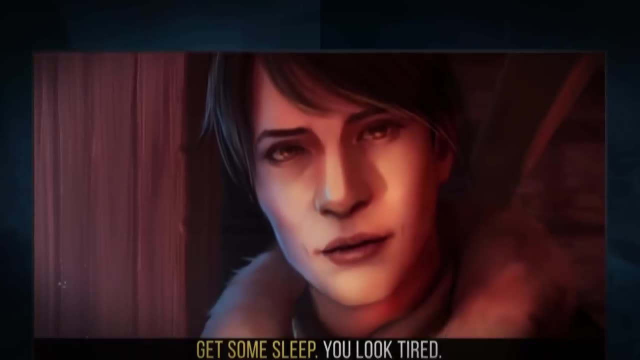 Someone Selene always thought was stubborn. Someone who's been stuck in a repeating loop of events. Someone who keeps being told that they need their rest, Just like the signs next to our cryopod tell us: Get some sleep. You look tired. 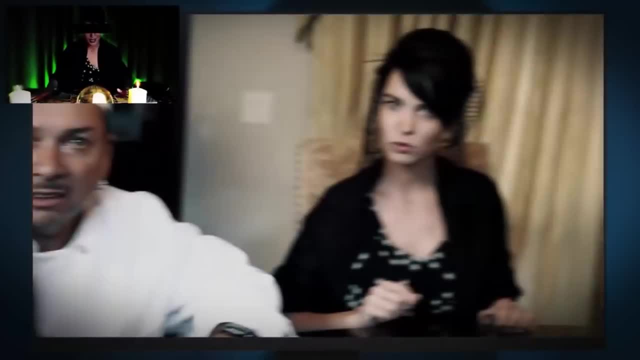 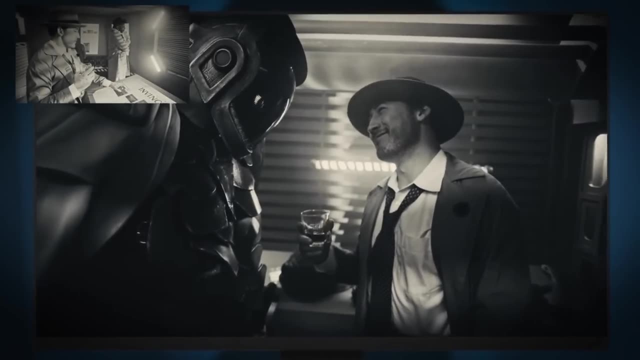 In fact, there's a lot of small stuff hidden in here too, Like how in Who Killed Markiplier, we get this line from the detective. Maybe I shouldn't have trusted someone so goddamn gorgeous. And in In Space we regularly hear things like: 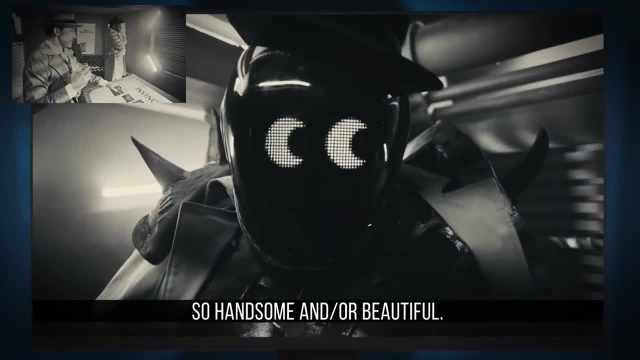 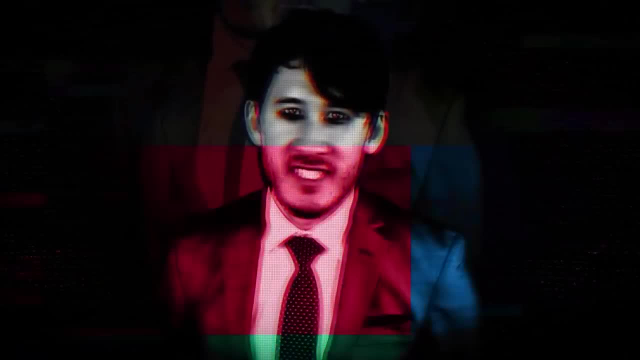 I could never lay eyes on a creature, so I could never lay eyes on a creature so handsome and or beautiful. We are once again considered attractive. This is why, Despite the fans crying out to see Darkiplier as a part of the series, he's yet to show up. 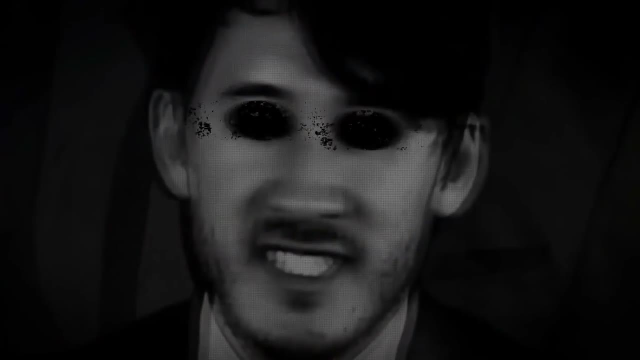 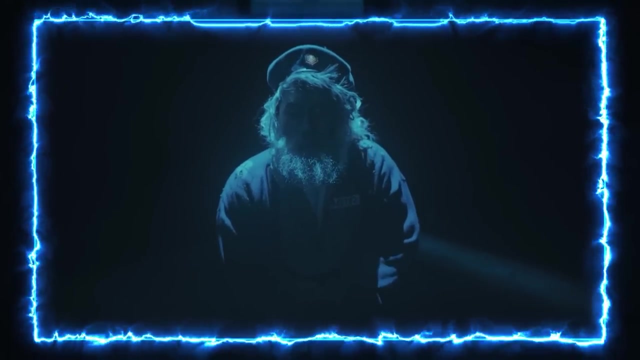 We've been inside his body the whole time. We've been looking through his eyes. It's also why actor Mark is so determined to beat us. Notice what happens during all the endings of part one. We're sent to a place outside the known universe. 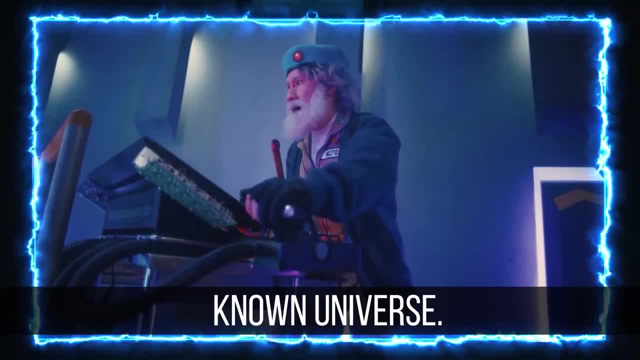 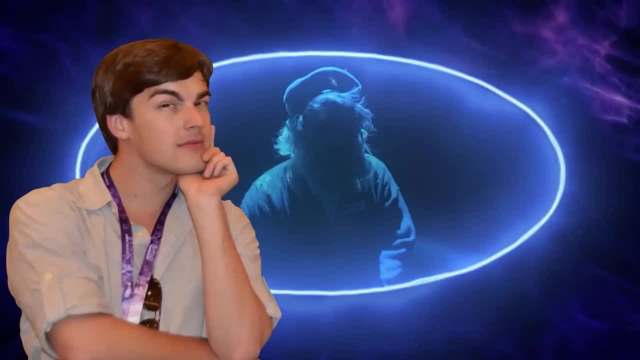 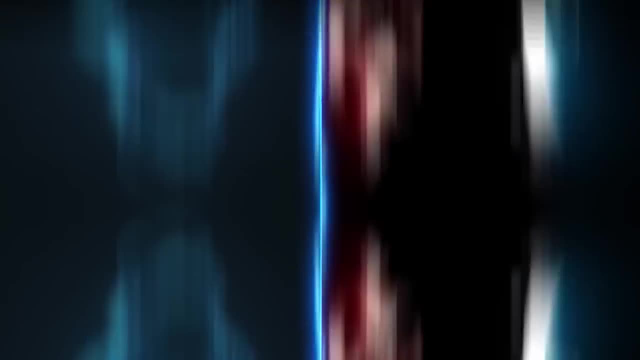 Be advised. designated location: outside known universe. I know That's the point: A black void with blue lighting. But is it just me, or does this look a little bit familiar Like, say, the black nothingness with blue that we see enveloping Damien in? Who Killed Markiplier? 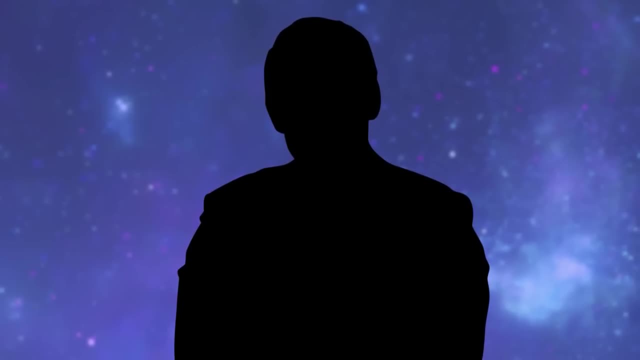 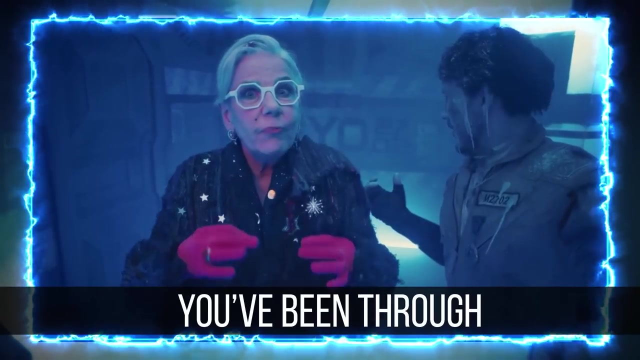 Or again in the ending of the video, Damien. The problem is we don't remember who we are. On multiple occasions we have Selene in the body of Doreen trying to jog our memories. It makes you feel like you've been through all this before. 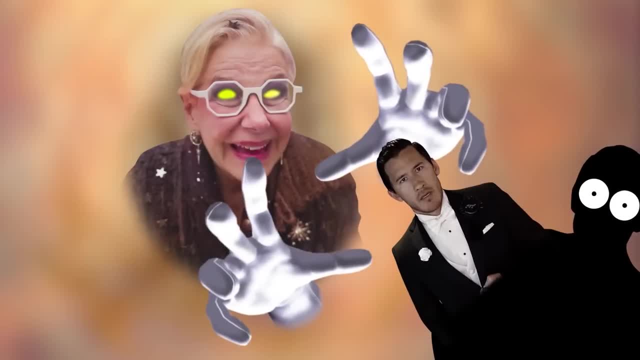 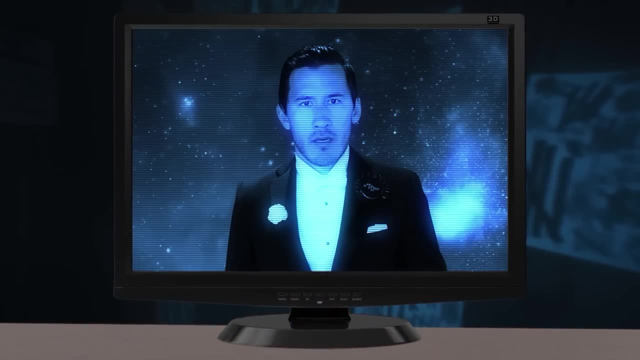 Do you understand dearie? She's trying to bring Damien to the surface. She's trying to remind him of who he is and what he has to do. And so now, with the universe being rebooted, I believe that's exactly what we're gonna start to see. 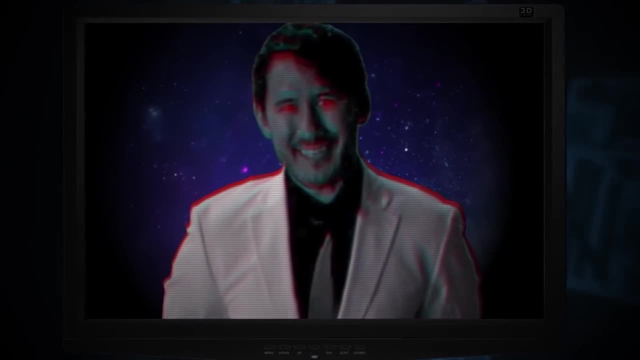 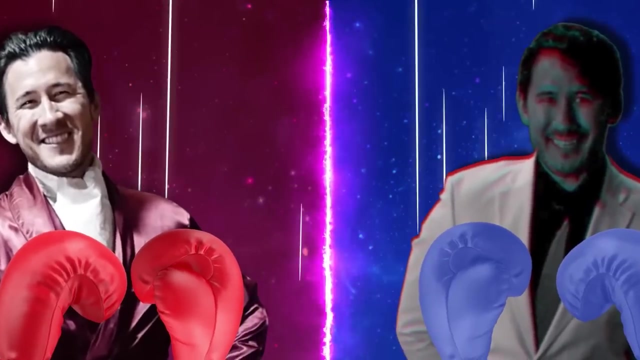 Damien beginning to remember Darkiplier becoming who he was meant to be. The reboot means the stage is now set for actor Mark and Darkiplier to have their final showdown. After all these years, they can finally put to rest this quest for revenge that's been keeping them going for so long. 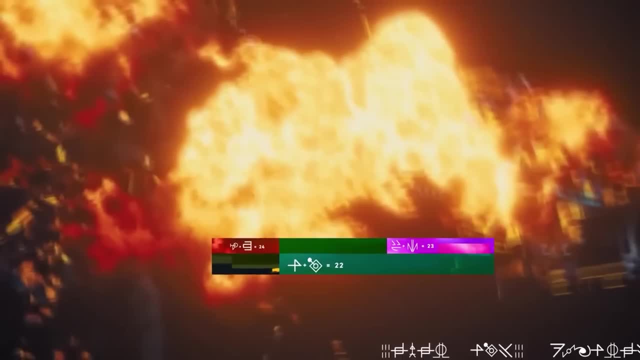 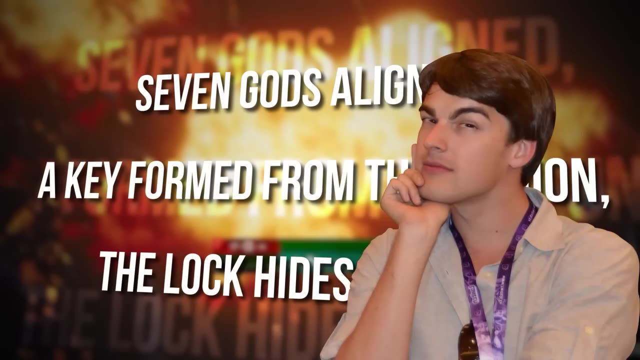 Recently, Mark released a teaser for part two full of codes that translated to quote: Seven gods aligned, A key formed from their union. The lock hides in time. Seven gods, you say. Remind me how many characters were in Who Killed Markiplier. 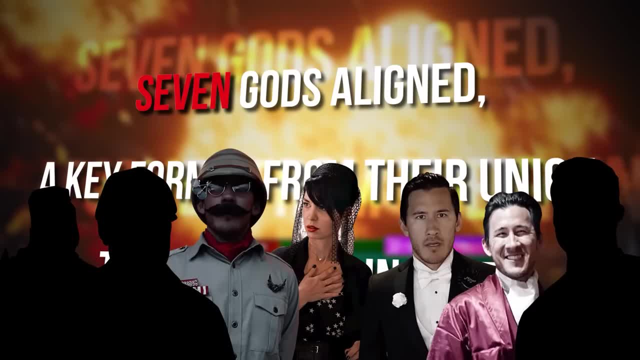 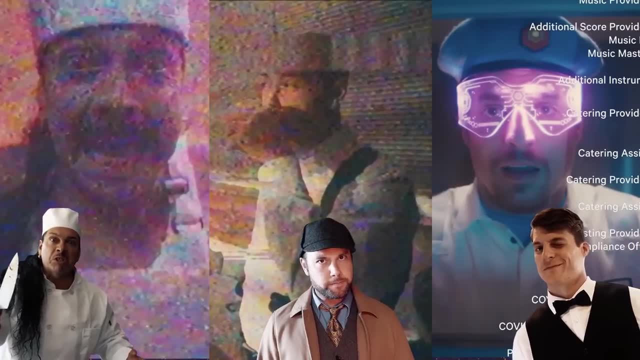 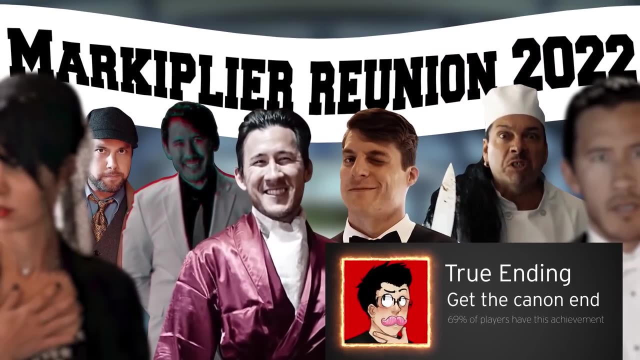 Oh yeah, seven: Selene, Damien Worfstache, actor Mark, even the detective, the chef and the butler, The last three of which appear as frame-perfect glitches in the endings of In Space. Basically, what I expect we're building towards is a reunion of all these characters, towards the true canon ending of the whole series.